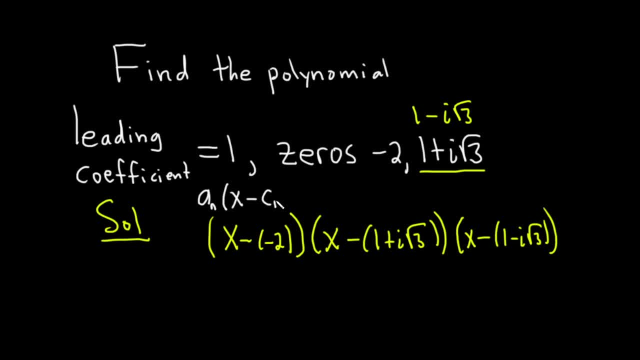 leading coefficient. you have some leading coefficient. you have some leading coefficient and it's x minus c1 times x minus c2 times dot, dot, dot, times x minus cn, where all of the c's are the zeros of the polynomial. It's really powerful. 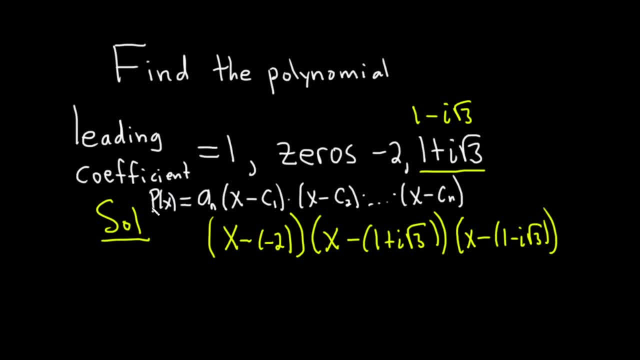 I'm just going to put a big p of x here to make it even more powerful. So big p is equal to all of this. So anytime you have a polynomial, you can always do this, you can always factor it, no matter what, And it's always x minus a zero, x minus a zero, And that's. 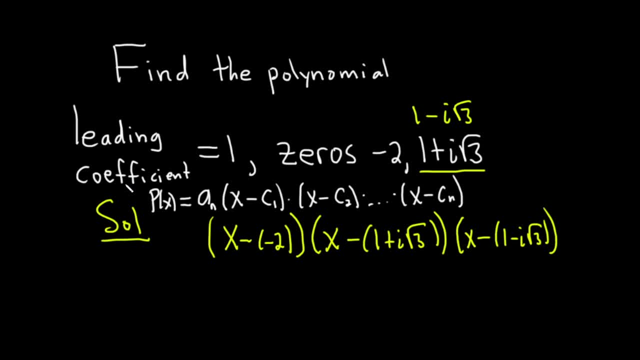 And that's the main idea in this problem. And then we're told the leading coefficient is 1.. So this, a sub n, is just 1.. So that's huge right, Because the fact it's 1 is going to make it much easier. 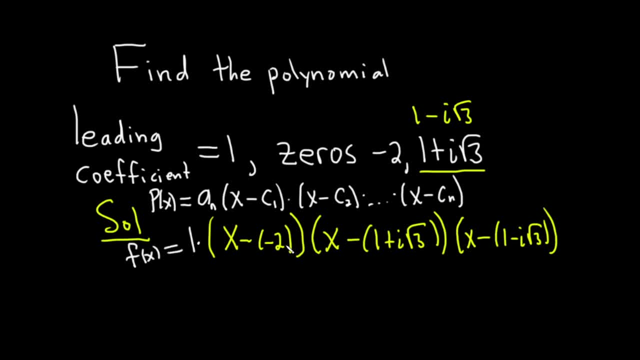 And so f of x is equal to this. Now we could leave it like this. However, I didn't write this down. The directions do say they want only real coefficients. Basically, they don't want to see any complex numbers in the solution. 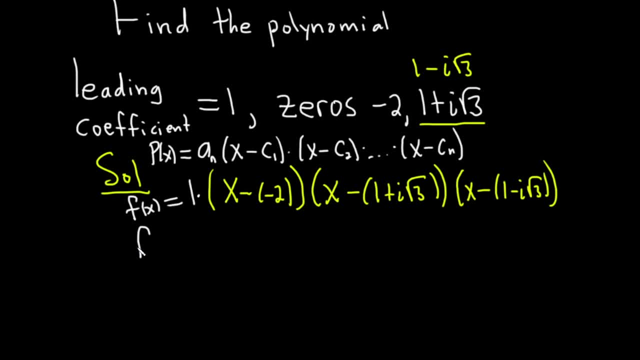 So we're going to have to take some steps to clear those. So we have f of x equals. Let's go ahead and write this as x plus 2.. And then here we can distribute the negative. There's a negative 1 here, right? 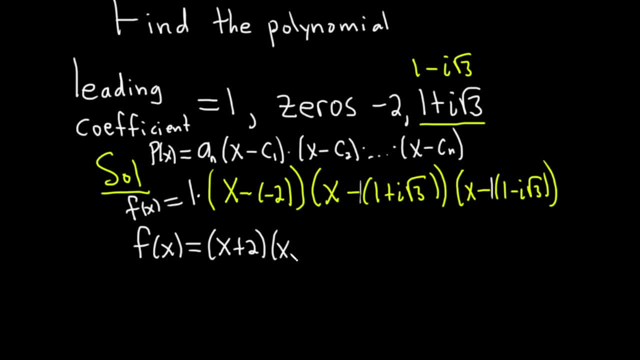 There's an invisible negative 1 here. This will be x minus 1.. And then let me write that a little bit bigger. And then negative 1 times the positive i square root of 3 is minus i square root 3.. And then here we have f of x equals. 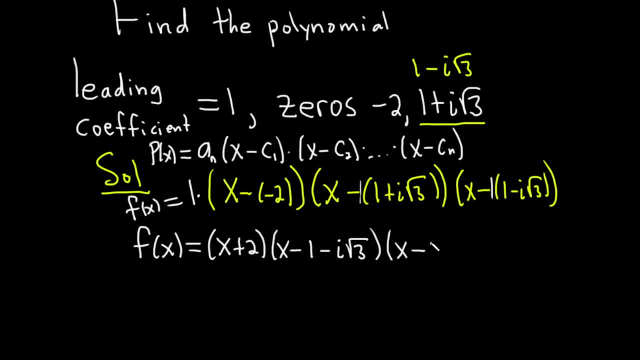 And then here it will be x and then negative, 1. And then negative and negative is positive. So plus i, square root 3.. Writing this again, we have f of x equals parentheses x plus 2.. Now here is where it gets really interesting. 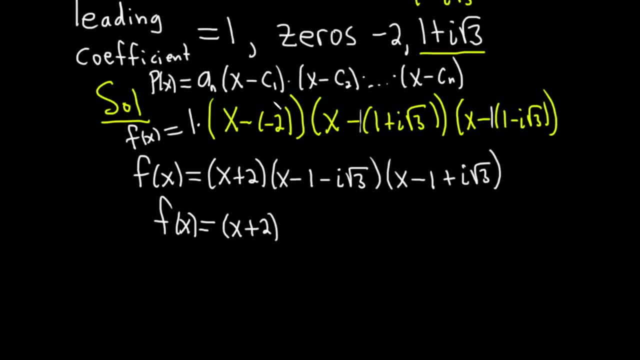 So what we're going to do now is simplify this, So I'm going to use a different color. So notice here that this is x, This is x minus 1.. And this is also x minus 1.. And so now what we're going to do is we're going to invoke a very powerful formula.